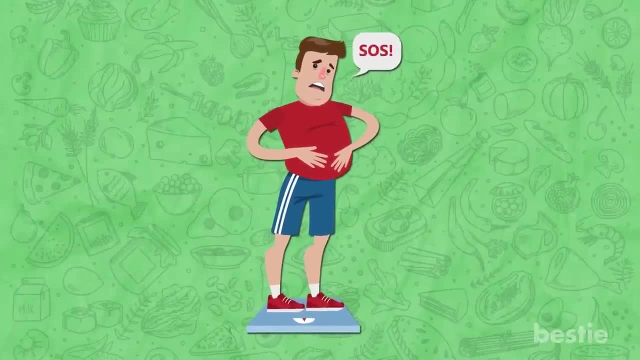 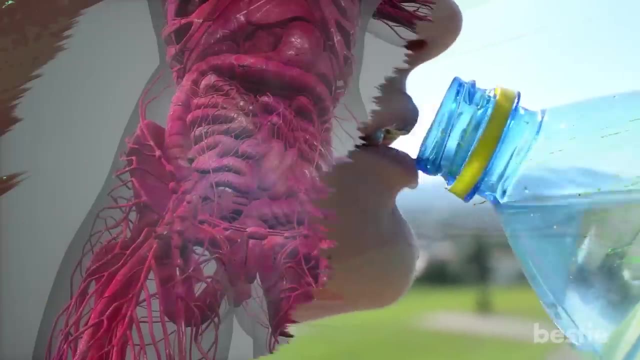 Even if you decide to go on a diet and not eat any more proper meals, you can still survive, Although you won't make it without water. For every organ of your body to work properly, it needs water. This liquid helps your brain function. 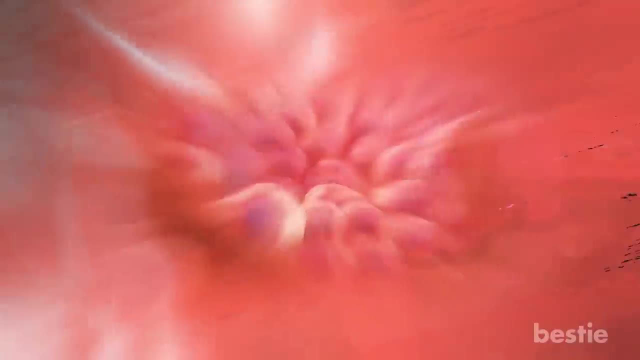 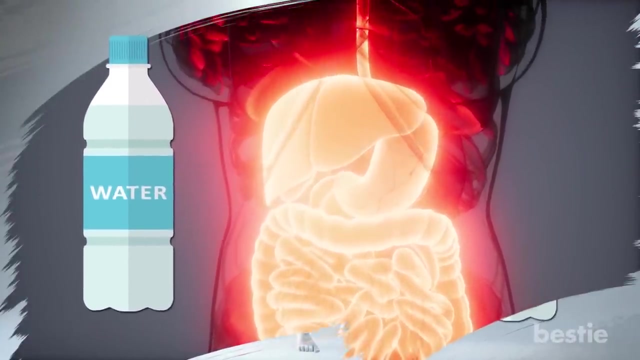 and cleanses your body of toxins. The cells in your body stay hydrated because of water. Apart from that, water also helps in the process of digestion. If you're someone who doesn't drink water regularly, you might find yourself constipated more often than not. 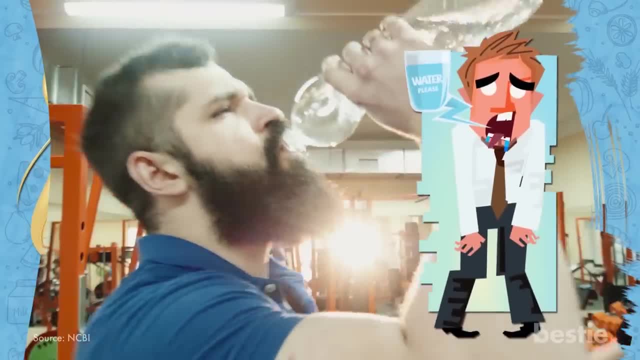 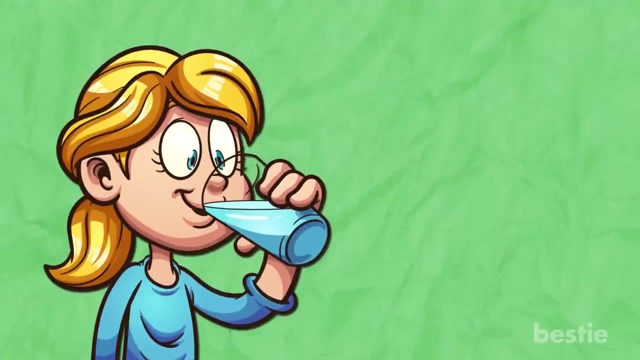 If you aren't drinking water properly, you'll end up becoming dehydrated. That's not a problem. It's not good for your body, as it can affect its mental and physical performance. Not drinking enough water can also make you feel tired and reduce your ability to concentrate. 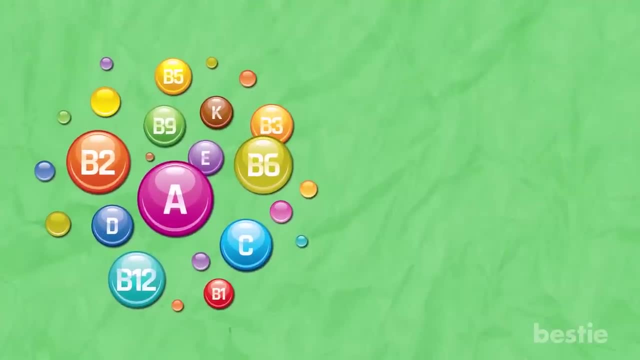 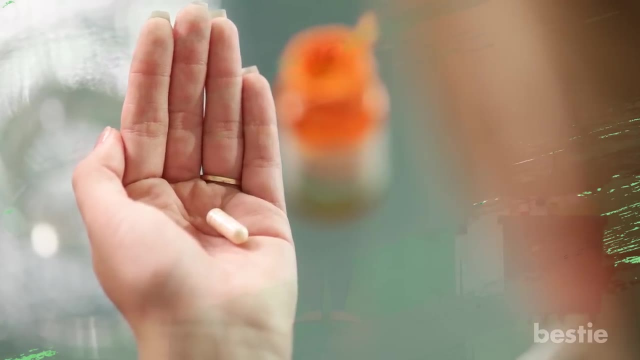 Vitamins. The basic function of these nutrients is to keep away diseases and keep you healthy. Without a healthy dose of vitamins, it would be difficult for your body to fight microorganisms, While there are about 13 types of vitamins that your body needs. 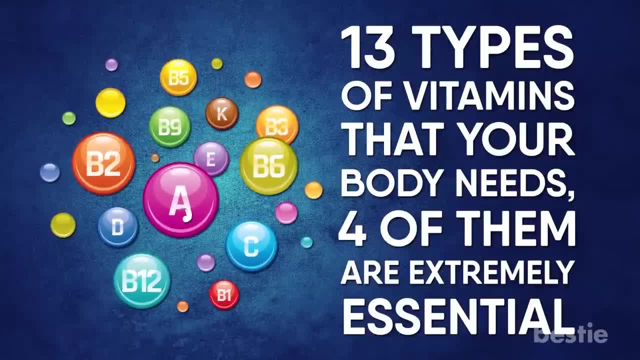 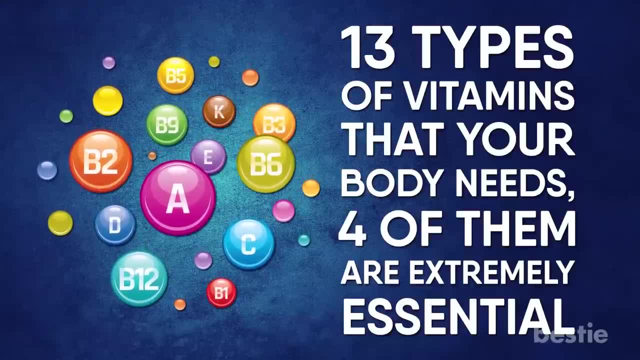 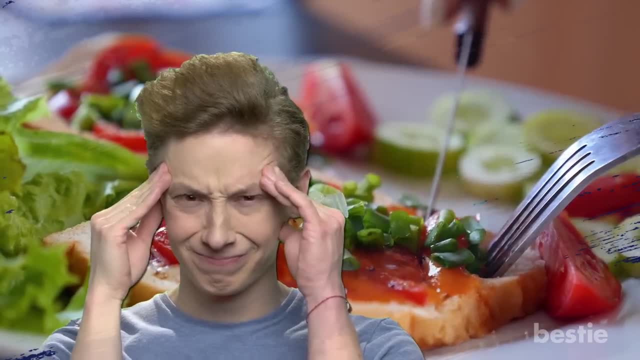 4 of them are extremely essential. These are vitamin A, B6, C and D. These 4 vitamins play an important role in your body. In case you aren't getting enough of these vitamins, you might face some problems. For example, lack of vitamin B6 can cause your blood pressure to lower uncontrollably. 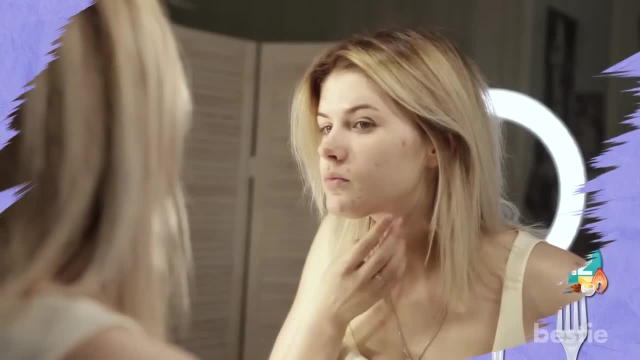 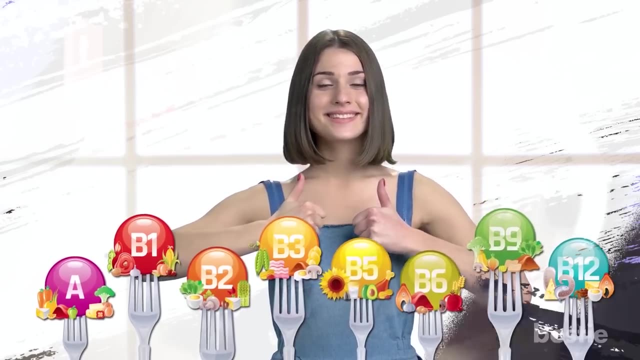 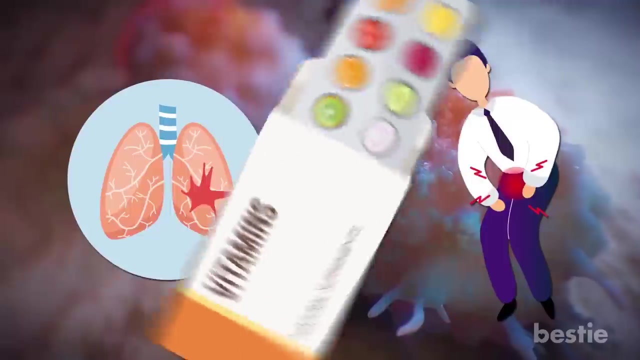 Similarly, lack of other vitamins may cause skin problems, vision problems and weakness. On the other hand, having enough vitamins in your body would mean you'll have a healthy immune system. The risks of getting lung and prostate cancer would also reduce with proper intake of vitamins. 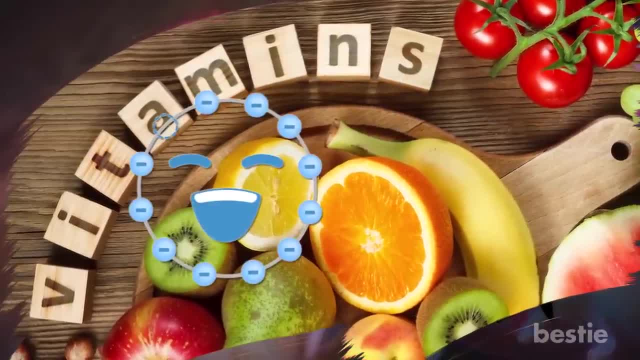 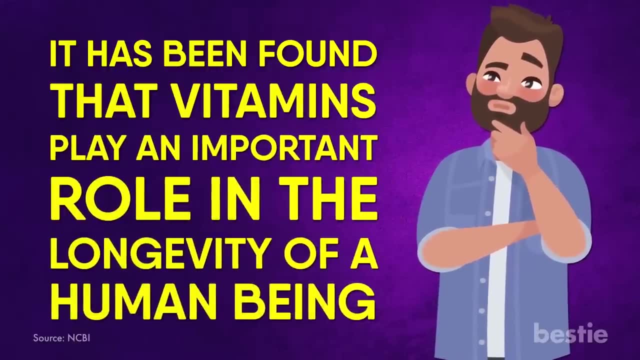 Additionally, vitamins also have high levels of antioxidants that are good for your body. What's more, it has been found that vitamins play an important role in the longevity of a human being. Protein- Protein. this is the nutrient that is called vitamin B1.. This is also one of the most important. 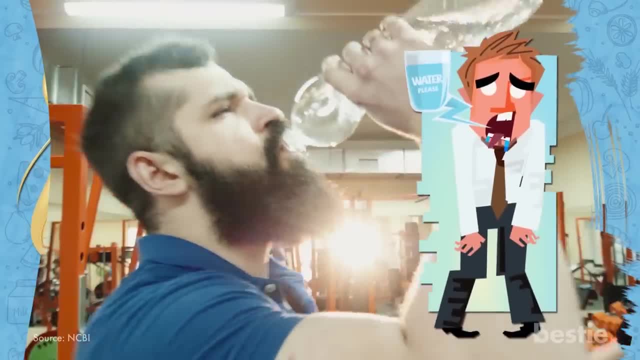 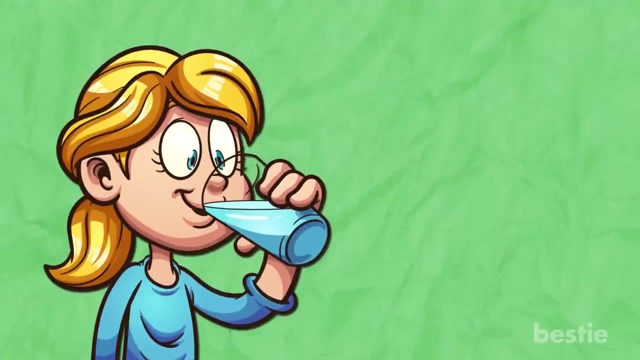 If you aren't drinking water properly, you'll end up becoming dehydrated. That's not a problem. It's not good for your body, as it can affect its mental and physical performance. Not drinking enough water can also make you feel tired and reduce your ability to concentrate. 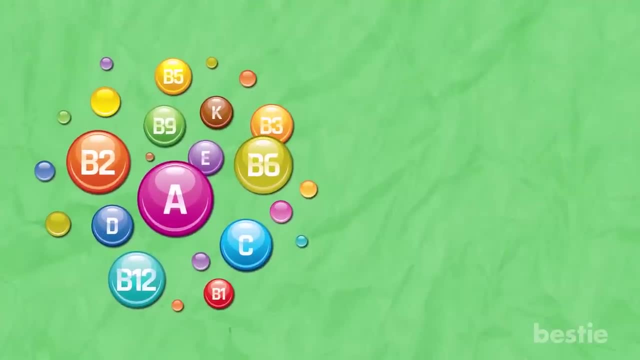 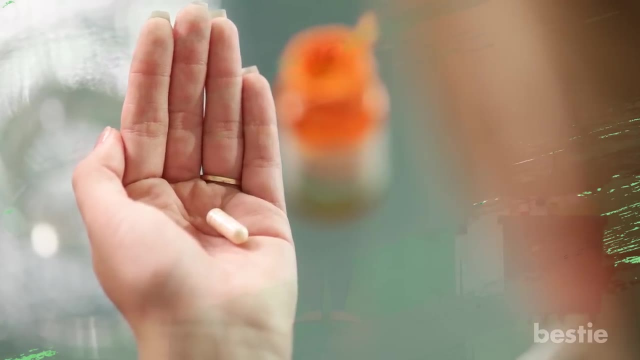 Vitamins. The basic function of these nutrients is to keep away diseases and keep you healthy. Without a healthy dose of vitamins, it would be difficult for your body to fight microorganisms, While there are about 13 types of vitamins that your body needs. 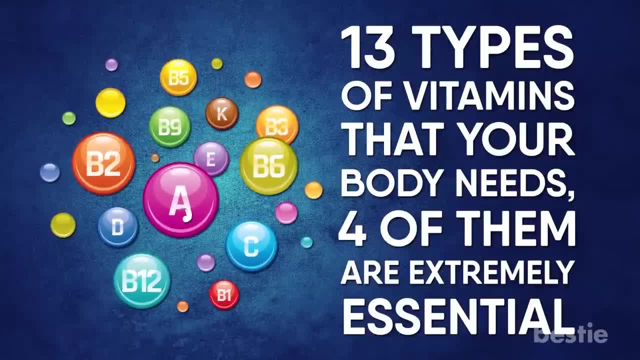 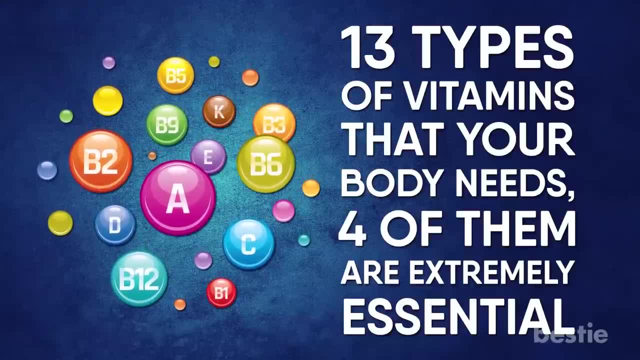 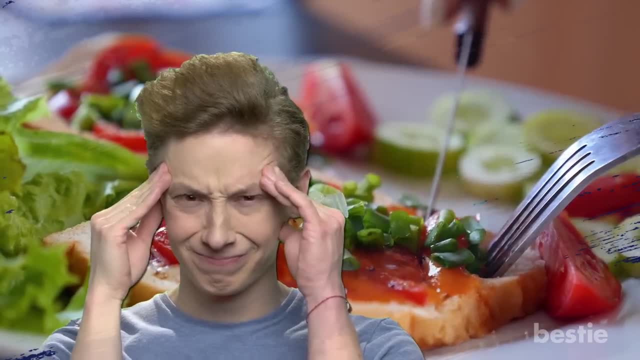 4 of them are extremely essential. These are vitamin A, B6, C and D. These 4 vitamins play an important role in your body. In case you aren't getting enough of these vitamins, you might face some problems. For example, lack of vitamin B6 can cause your blood pressure to lower uncontrollably. 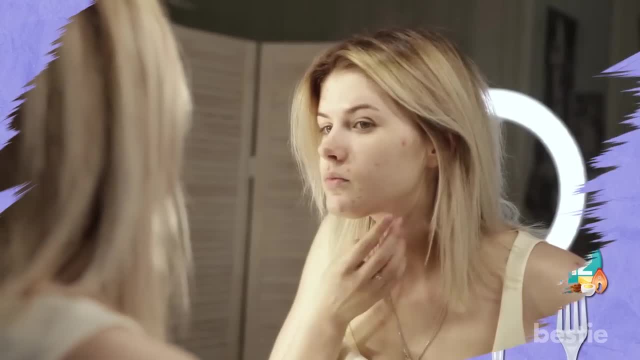 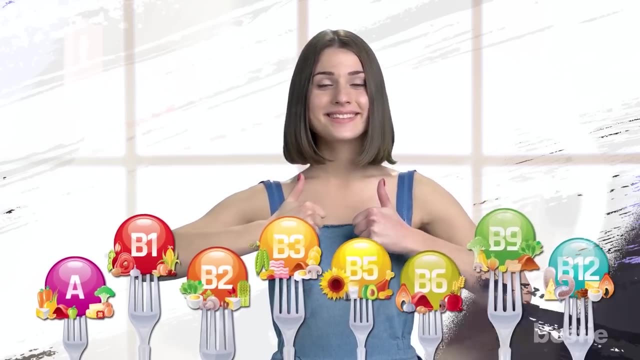 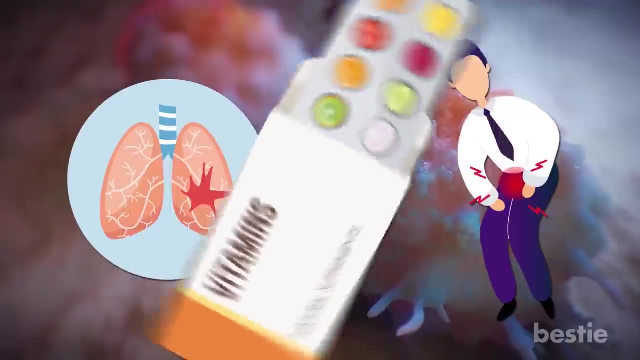 Similarly, lack of other vitamins may cause skin problems, vision problems and weakness. On the other hand, having enough vitamins in your body would mean that you will have a healthy immune system. The risks of getting lung and prostate cancer would also reduce with the proper intake of vitamins. 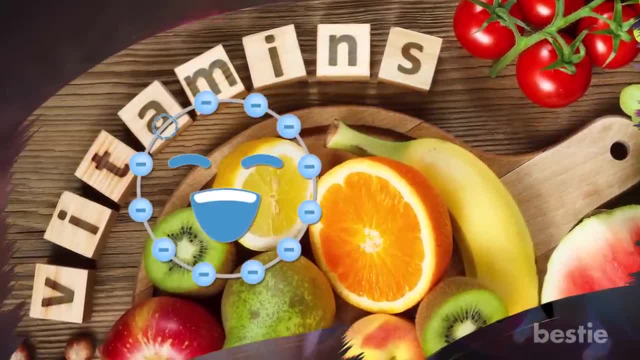 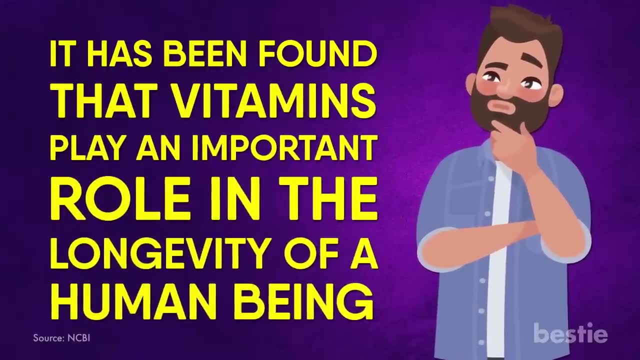 Additionally, vitamins also have high levels of antioxidant properties that are good for your body. What's more, it's been found that vitamins play an important role in longevity of a human being. Protein, It's the nutricient that helps the body to go from being full to being full of vitamin C. This is 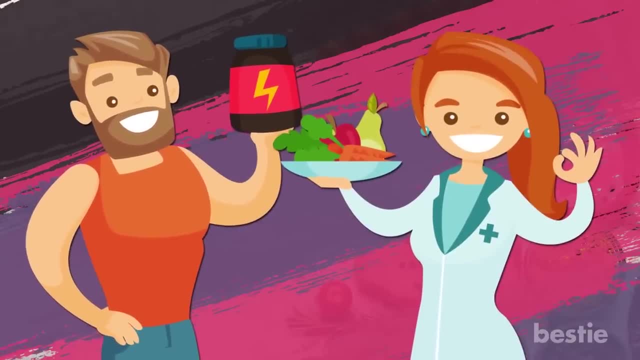 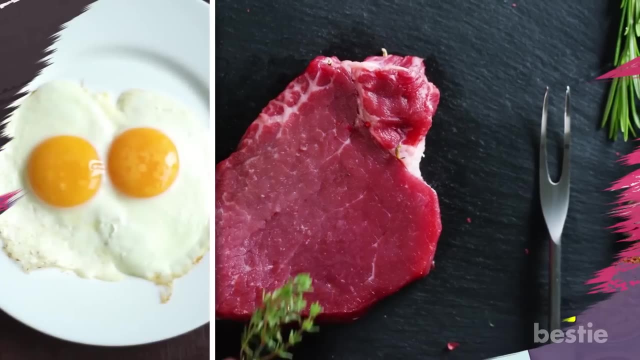 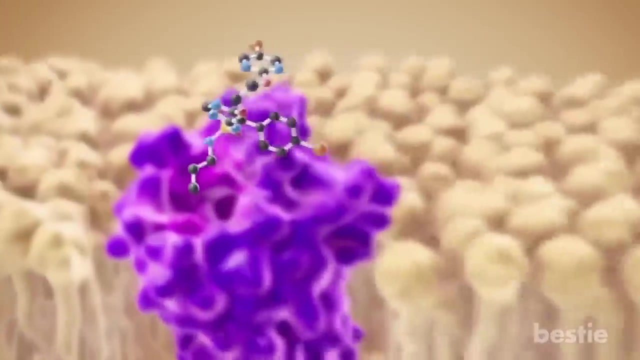 the nutrient that gets the most hype. Go to any nutritionist and they will suggest a lot of food items for the proper intake of protein. These include meat, eggs and some grains. So why is protein so popular? Well, protein is the building block of your body. No, we. 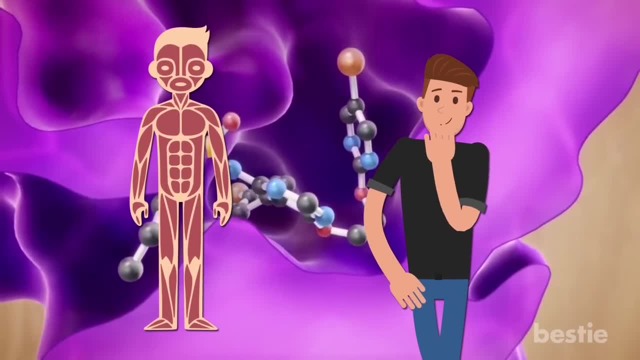 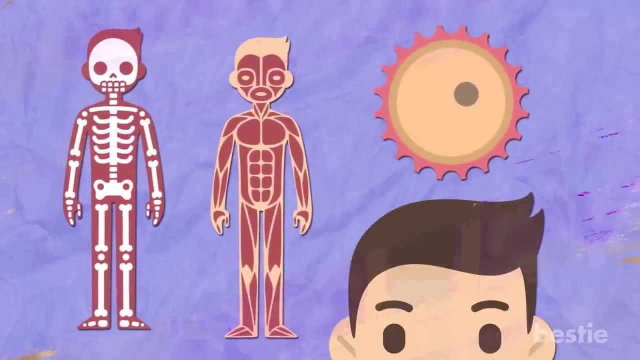 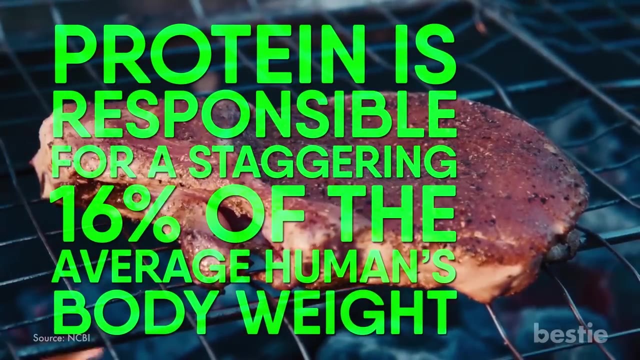 don't mean just muscles. We are talking on a deeper level. Whether it's your bones, muscles, skin, hair or even the cells in your body, everything contains protein. In fact, protein is responsible for a staggering 16% of an average human's body weight. Even 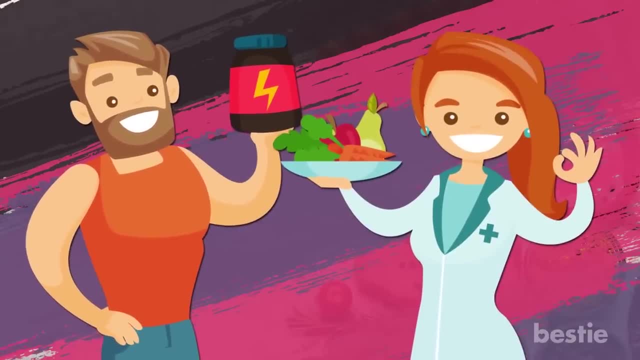 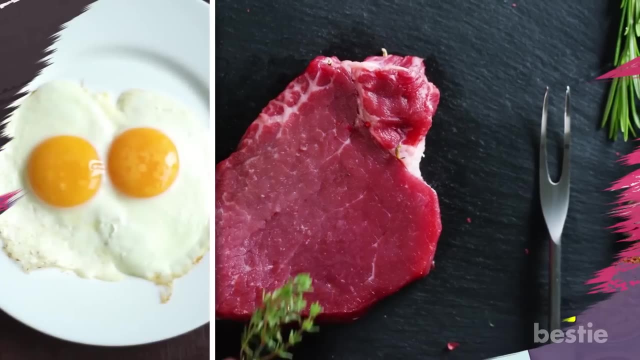 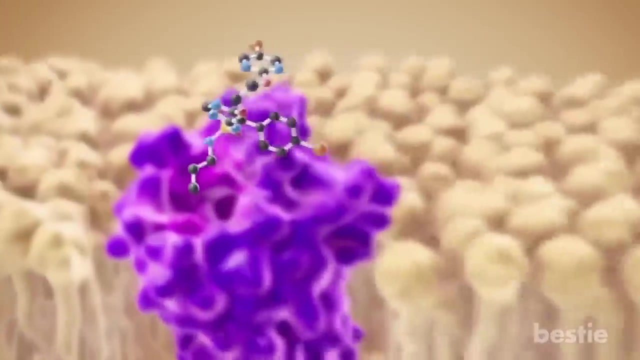 the nutrient that gets the most hype. Go to any nutritionist and they will suggest a lot of food items for the proper intake of protein. These include meat, eggs and some grains. So why is protein so popular? Well, protein is the building block of your body. No, we. 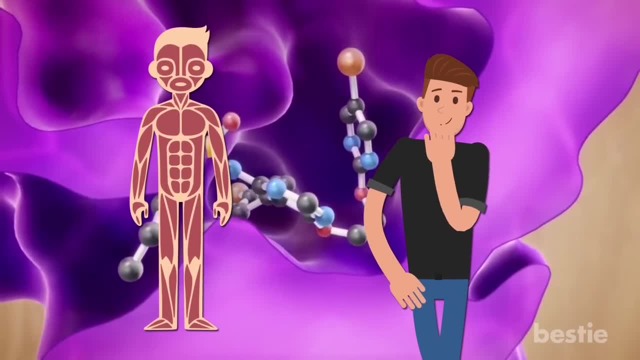 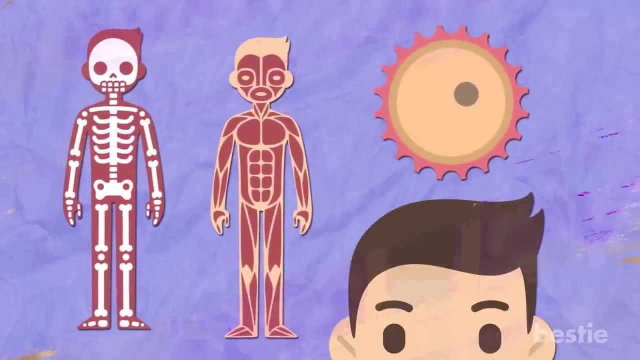 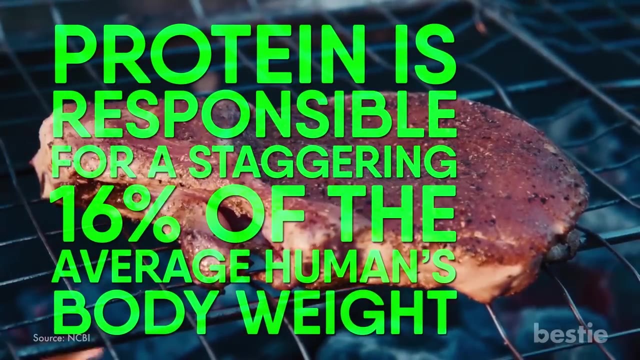 don't mean just muscles. We are talking on a deeper level. Whether it's your bones, muscles, skin, hair or even the cells in your body, everything contains protein. In fact, protein is responsible for a staggering 16% of an average human's body weight. Even 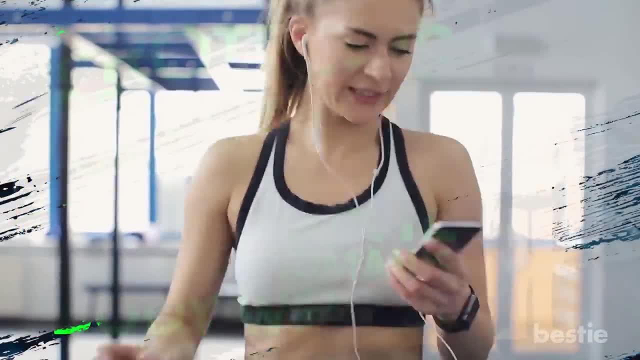 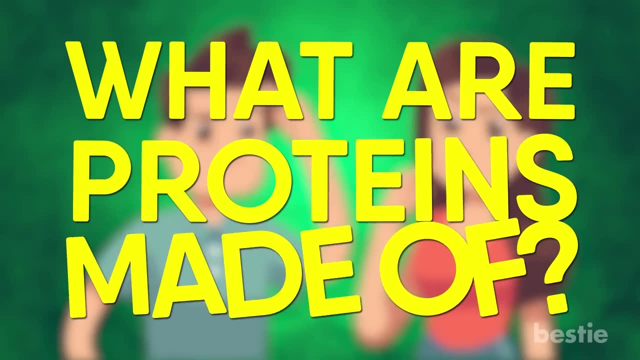 your hormones and antibodies are composed of proteins. In other words, it would be very difficult to live without this nutrient. This begs the question: what are proteins made of? Well, the answer is fairly simple: They are made up of different types of proteins. They are made up of different types of proteins. 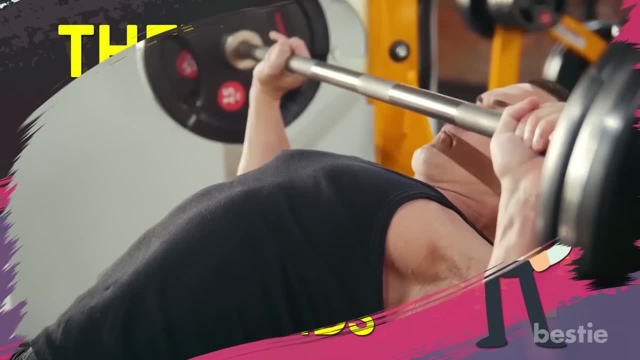 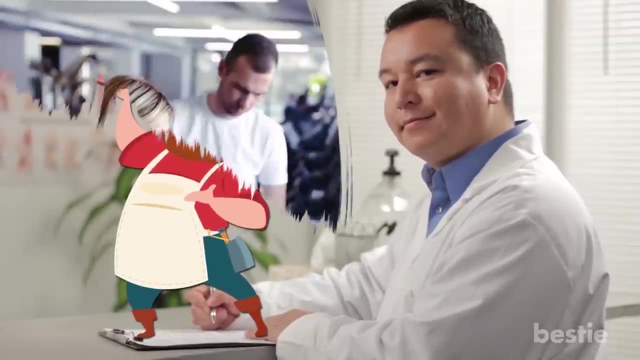 They are made up of different types of amino acids. Your body needs protein so that it can function properly. This is why your nutritionists always stress that you have a lot of protein in your diet, even if you are looking to lose weight. So the next time they ask you to have 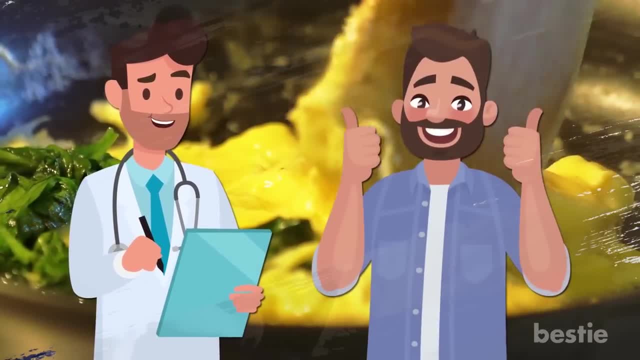 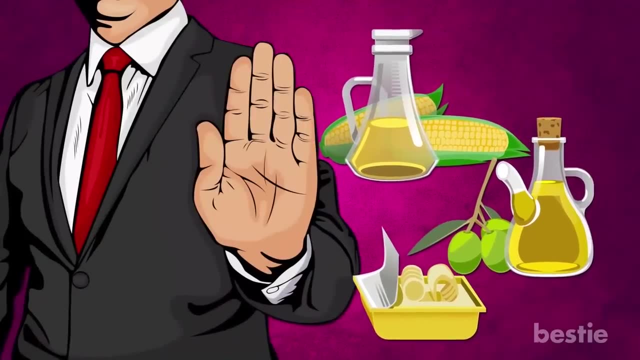 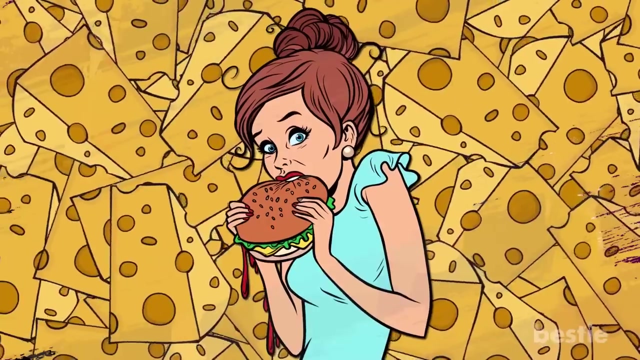 scrambled eggs at breakfast. take the advice. They only want what's good for you. Fats, Yes, the nutrient that you want to avoid. Well, maybe you shouldn't avoid it so much, after all, Of course, An excessive amount of fats may be dangerous for your body. Too much fat can cause problems. 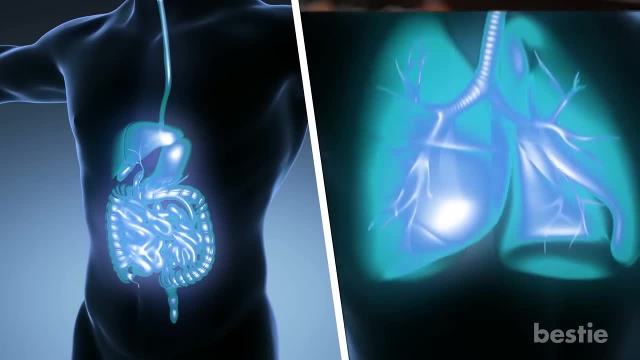 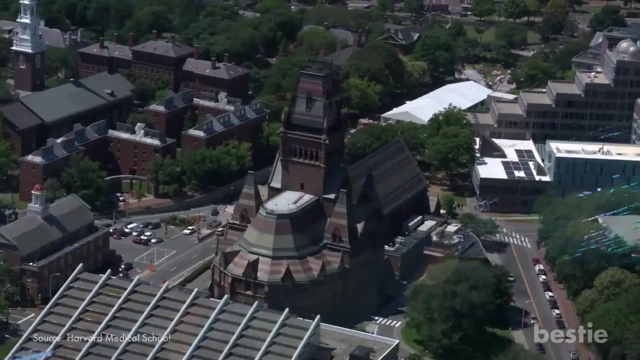 for our blood pressure levels and heart, as well as our digestive and respiratory systems. So why are we saying you shouldn't avoid fats? Well, according to a study at Harvard Medical School, it was found that fats help the absorption of other nutrients On top. 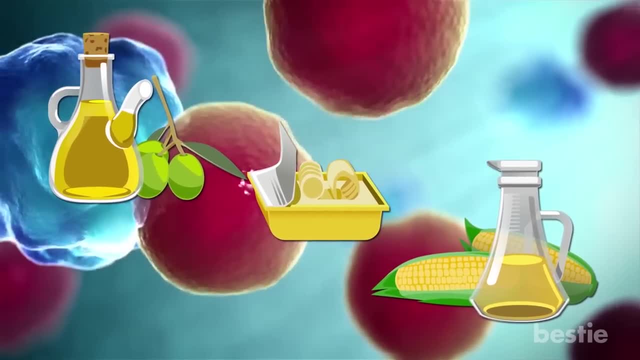 of that, fats play an important role in cell building. If that wasn't enough to convince you, the study also showed that fats can help the absorption of other nutrients. If you're not sure what you're talking about, check out our other videos on how to avoid fats. 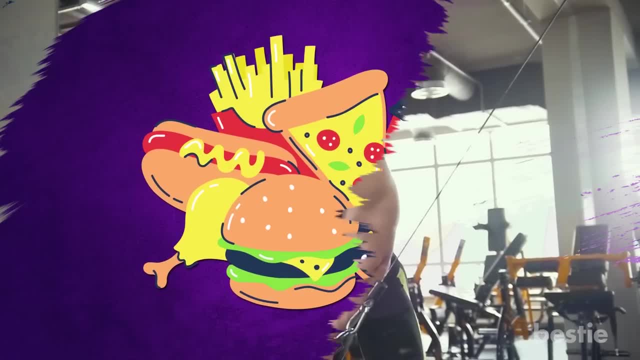 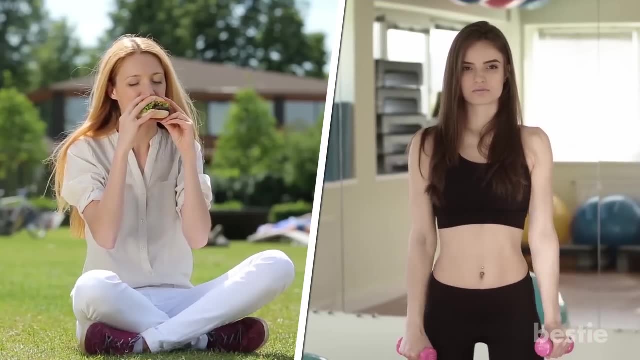 So what are the benefits of fats? Fats help to improve your muscle movement. While you might want to avoid fat because of high amounts of calories, it would be better if you ingest it and then burn those calories instead. Additionally, if you can consume fats on a controlled basis and burn calories, 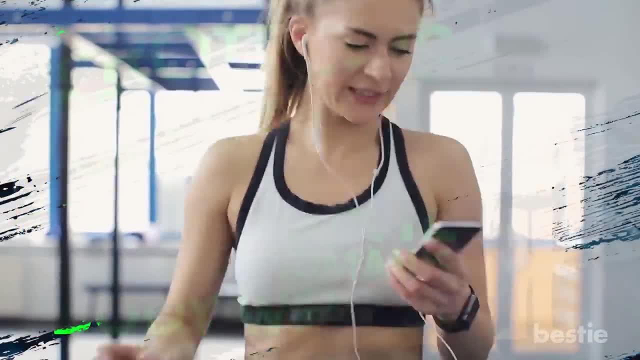 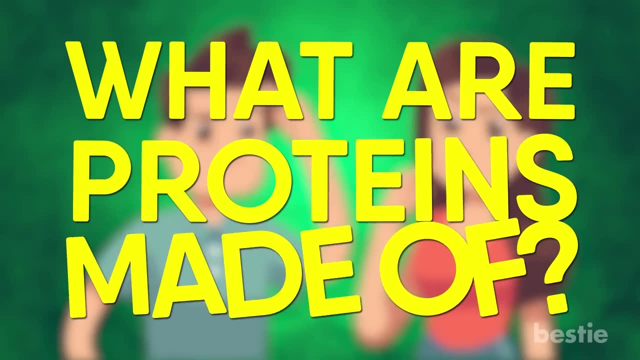 your hormones and antibodies are composed of proteins. In other words, it would be very difficult to live without this nutrient. This begs the question: what are proteins made of? Well, the answer is fairly simple: They are made up of different types of proteins. They are made up of different types of proteins. 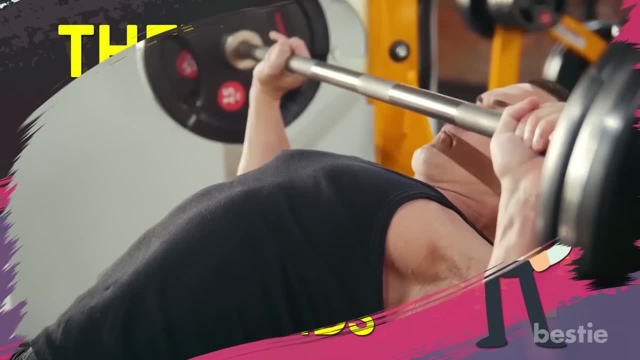 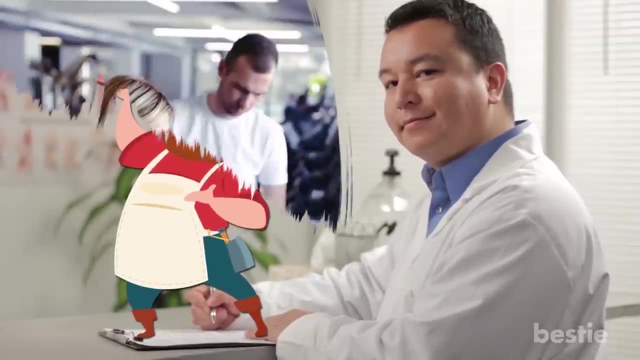 They are made up of different types of amino acids. Your body needs protein so that it can function properly. This is why your nutritionists always stress that you have a lot of protein in your diet, even if you are looking to lose weight. So the next time they ask you to have 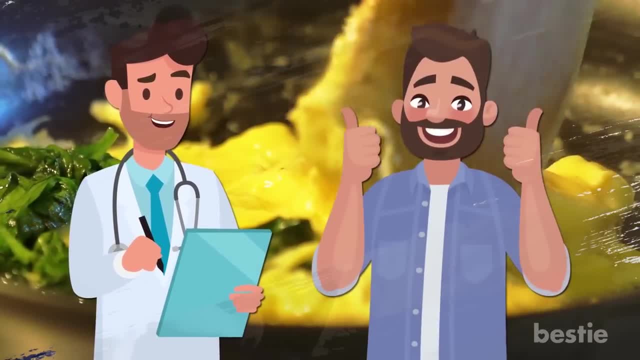 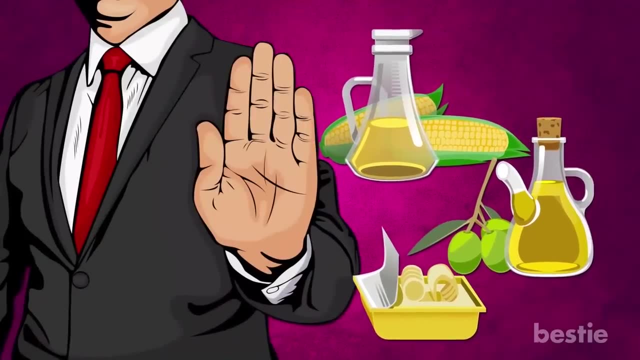 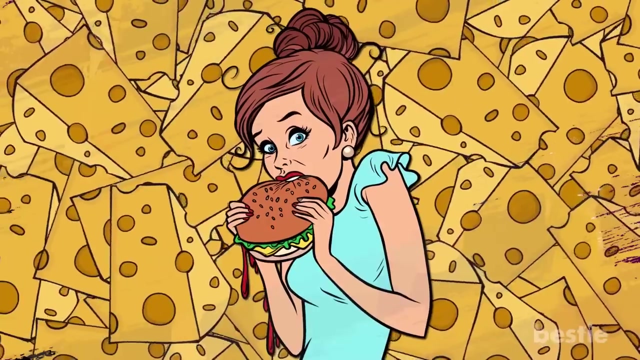 scrambled eggs at breakfast. take the advice. They only want what's good for you. Fats, Yes, the nutrient that you want to avoid. Well, maybe you shouldn't avoid it so much, after all, Of course, An excessive amount of fats may be dangerous for your body. Too much fat can cause problems. 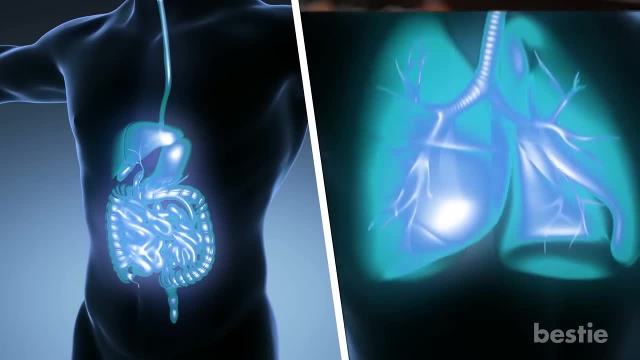 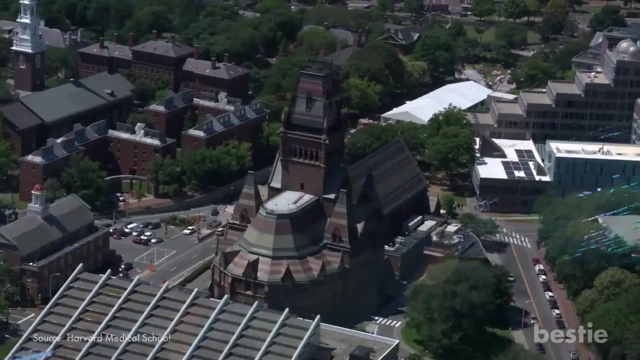 for our blood pressure levels and heart, as well as our digestive and respiratory systems. So why are we saying you shouldn't avoid fats? Well, according to a study at Harvard Medical School, it was found that fats help the absorption of other nutrients On top. 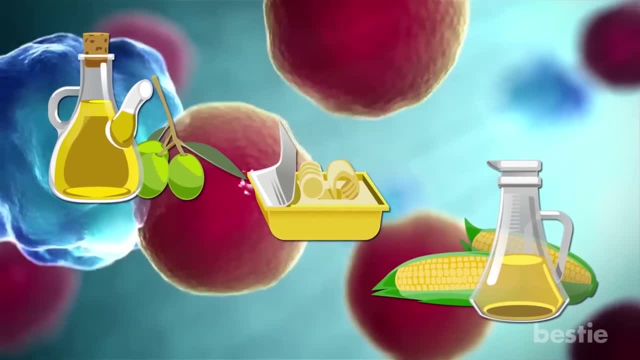 of that, fats play an important role in cell building. If that wasn't enough to convince you, the study also showed that fats can help the absorption of other nutrients. If you're not sure what you're talking about, check out our other videos on how to avoid fats. 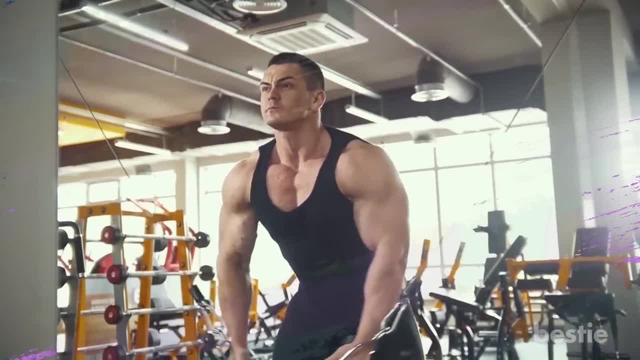 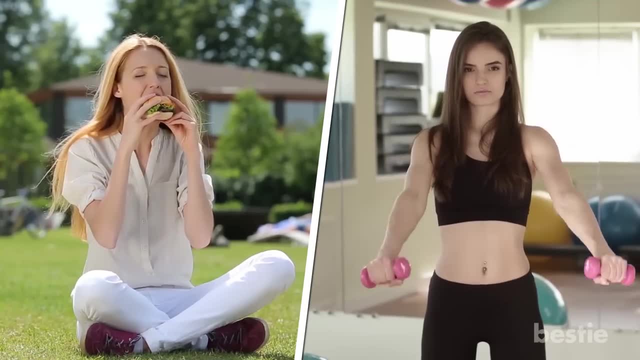 The study also showed that fats help to improve your muscle movement. While you might want to avoid fat because of high amounts of calories, it would be better if you ingest it and then burn those calories instead. Additionally, if you can consume fats on a controlled basis, 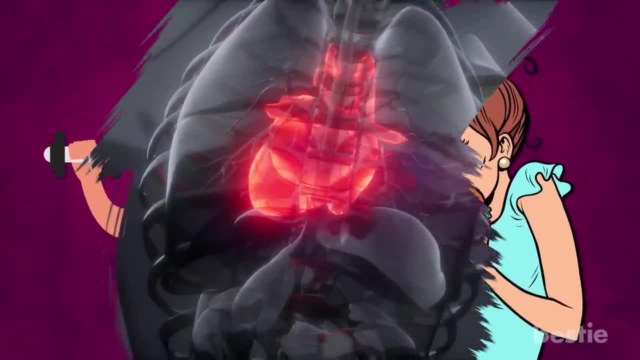 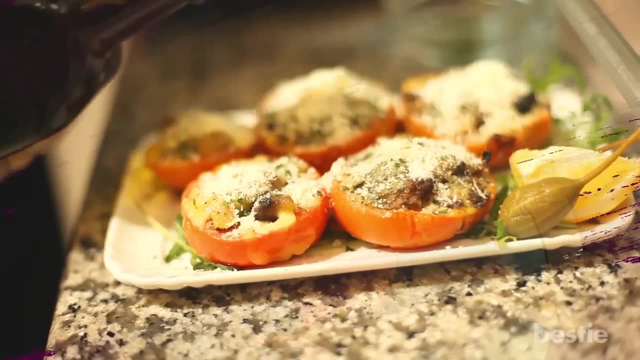 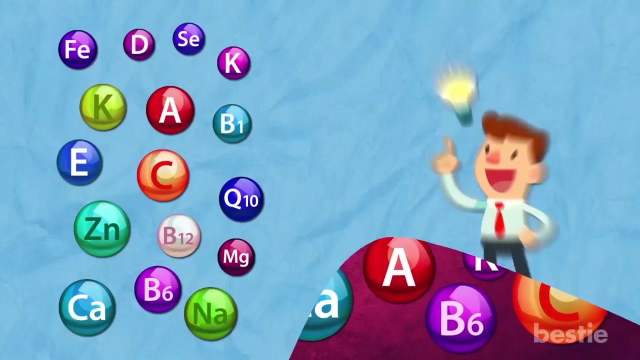 and burn calories, it will decrease the risk of heart diseases. More importantly, you will have a lower chance of getting type 2 diabetes. It had also been speculated that controlled intake of fat improves brain function. Minerals: When we talk about minerals for our body, the first thing that might come to mind is: